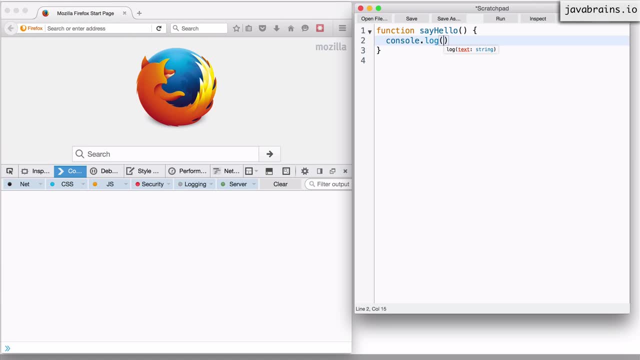 So here I'm going to print a simple consolelog- hello right, Very simple function which contains one line of code which prints something to the console. And now the way to execute the function is by using the name of the function, with the same open, close braces, Okay, And 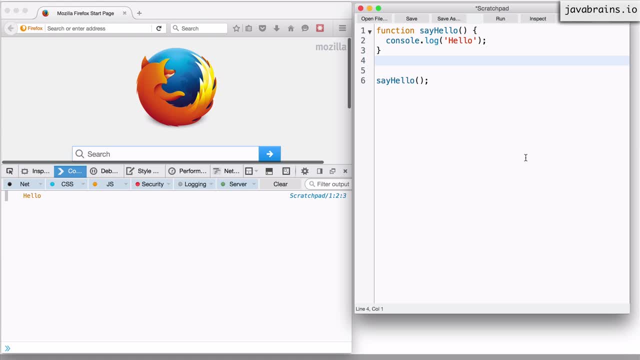 if I were in parentheses. I'm sorry. If I were to execute this reload and run, I'm see hello being printed, so i'm declaring a function and i'm calling it using its name. all right now, this is what results in the hello being printed over here when the javascript interpreter 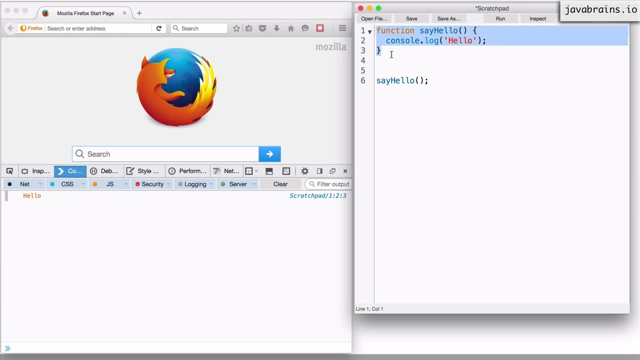 runs. it executes line one and says, okay, there is a function declaration. it registers this function, but it does not print anything to the console. the execution comes all the way to line six and this is where the, the function, is called, and that's where the control jumps back to line two. 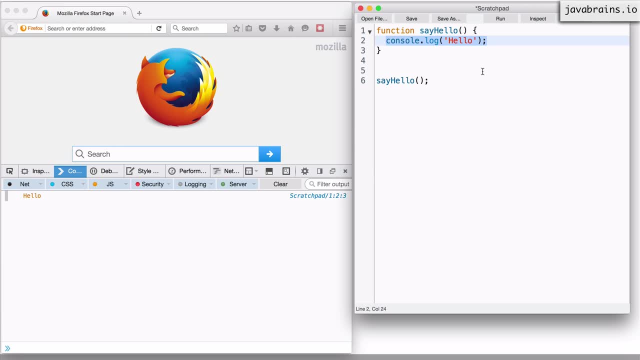 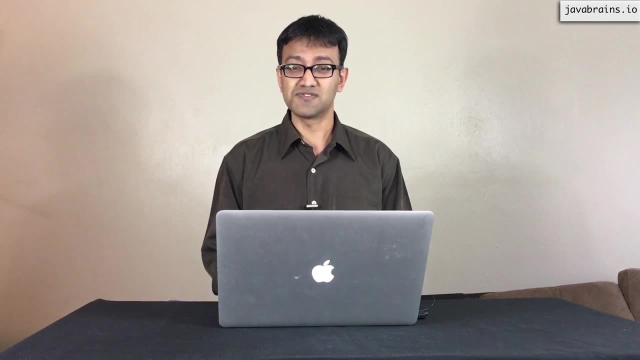 and prints the value to the console again. this is simple function concepts, which is, you know, kind of common across multiple programming languages. this shouldn't be much of a surprise to you guys. all right, so functions can also take in arguments. like i said, if i were to say hello to a person and 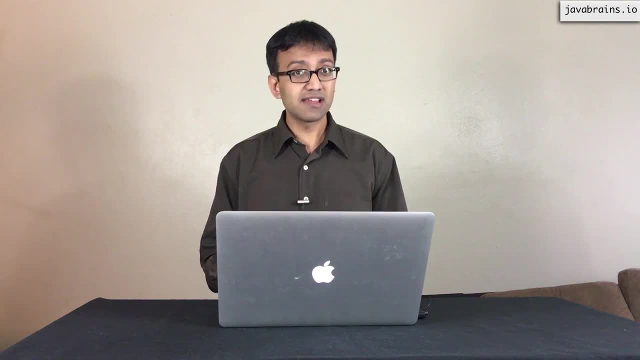 i want the person's name to be passed in as an argument, i can declare the function as some kind of a function. and if i want to say hello to a person and i want the person's name to be passed in as an argument, i can declare the function as some. 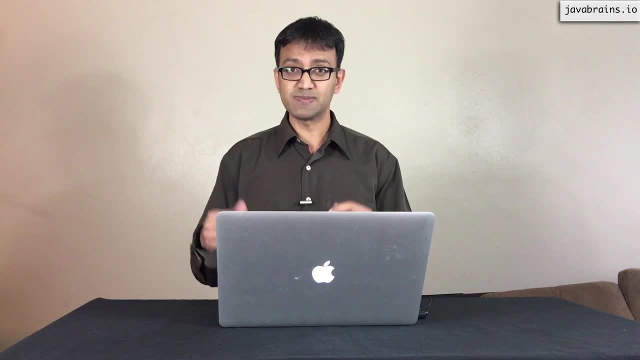 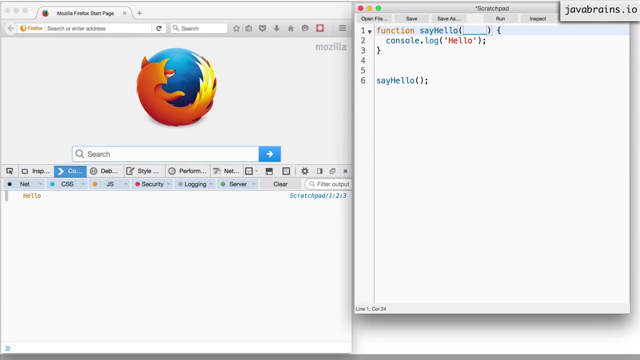 thing that accepts arguments, and then, when the argument is passed, i can use that argument in my logic. so debate, the way to create and declare an argument to the function is typically in, even in other programming languages, it is when you write something here, between these parentheses, which indicate what your parameters for the function are going to be: c plus plus java, they all. 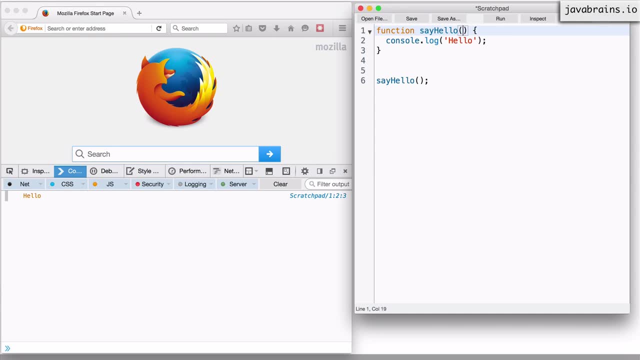 have the same concept. so typically in those languages what you would do is you give the data type and the variable name which is going to contain the value that somebody who is calling it would have passed. so it would be something like int a and then float b and all that stuff, but in javascript. 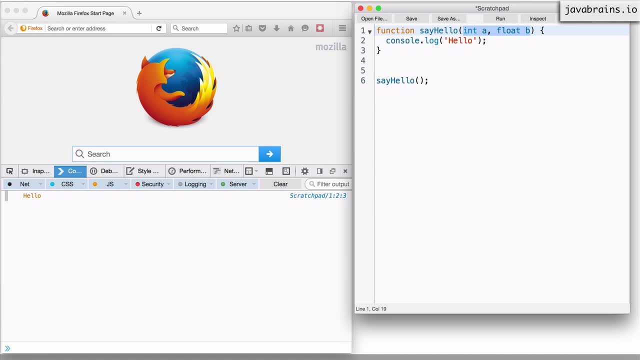 we don't have these kind of typed variables, right, everything is a war. so you don't have int and float and double and all that. so rather than have var a and then var b, the language designer start by simply add var, just skip it, so you don't have to declare. 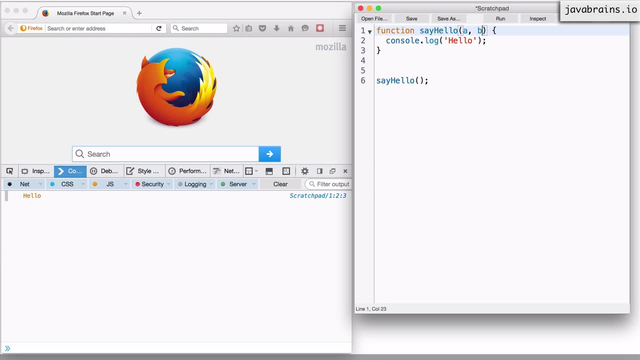 the type or even declare it as a water. you just send the list of arguments as, uh, you know, a list of variables, comma separated, and those get the right value. so in this case i just want to take one value, which is the name. so i'm just going to say name, okay. so no var name, no string name, just. 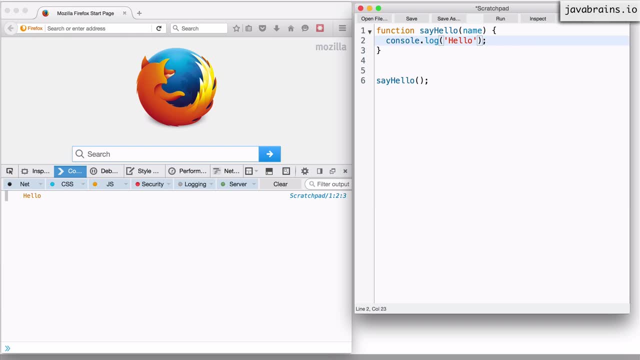 name now that now that i have name here, i can say hello to that person. so i'm just going to use the string concatenation here and then. then i say hello name. and now, if i were to call this function with a name value, which is again. 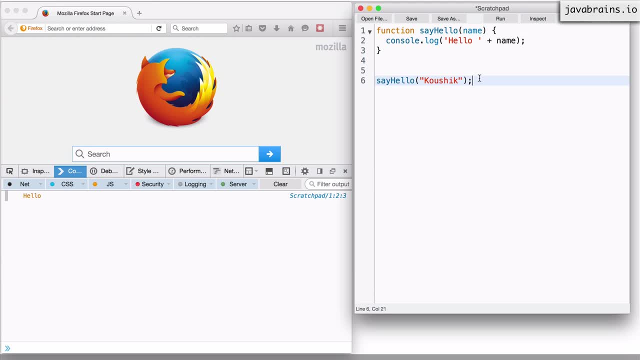 sending the actual value in the parentheses. let's say, i want to say hello to myself. now i can right click and run and it is going to say hello kaushik. because kaushik is the value, the string value, that is sent to the function when the function executes. 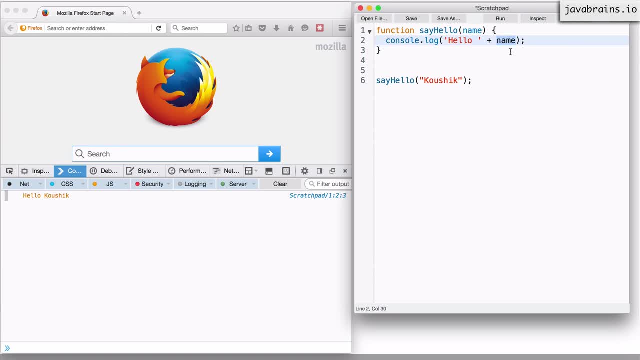 name is going to be a variable which contains a value, which is the string. kaushik. send parameters to functions. you can have multiple parameters as well. The way to send multiple parameters is again using comma separated values here, And then you know. 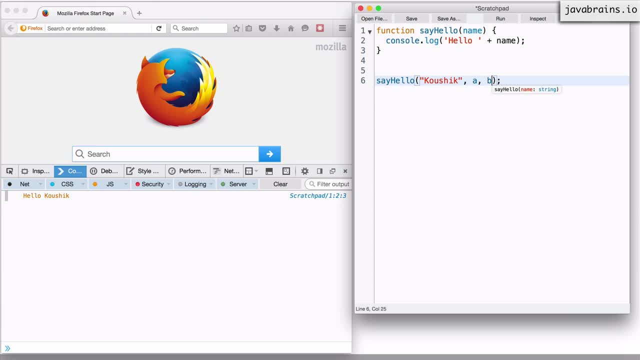 you can say multiple parameters over here, And then you can accept the right parameters over here again, comma separated. So let's let me add one more argument And I'll show you some weird thing that JavaScript does. For now everything is more or less it makes sense. 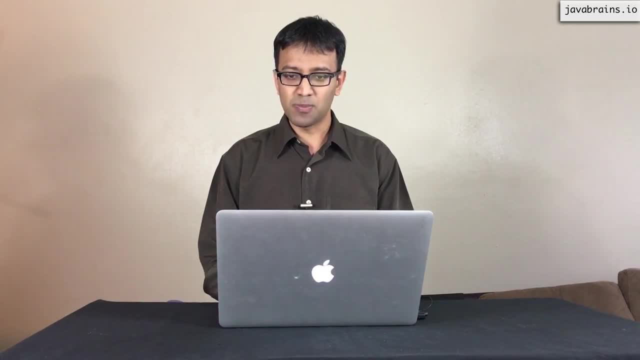 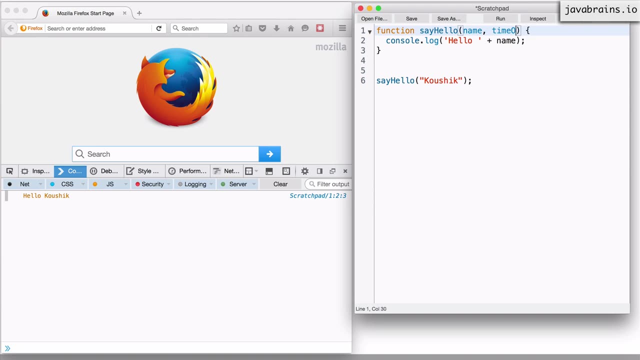 right, I hope it does. So let me add one more parameter, which is, let's say, time of day. Okay, and I'm just going to print that here. I'm just accepting another argument and then printing the message time: okay, So I'm just going to print that here, And I'm just going to print that here, And I'm just.